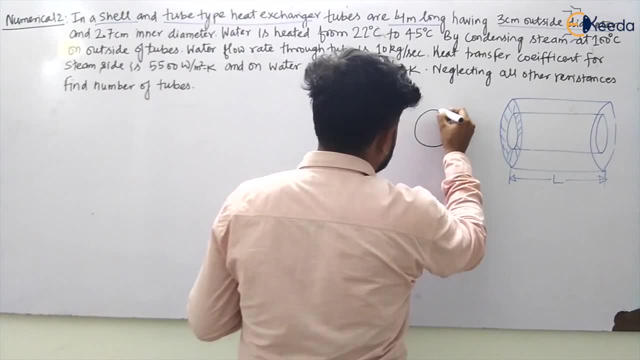 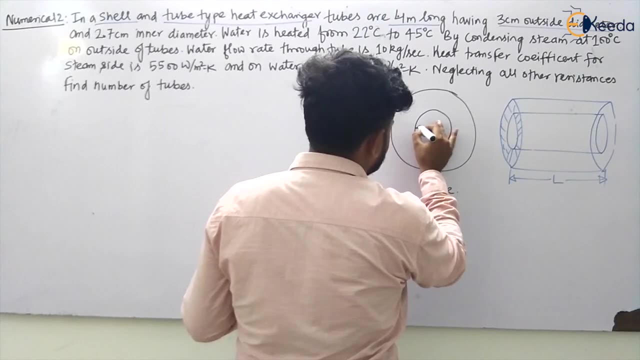 given. So if I will make this diagram to be like this, so this will be your inner diameter for a tube. Let us think this is your tube and they have given some inner diameter di and they have also given some outer diameter d, not values. 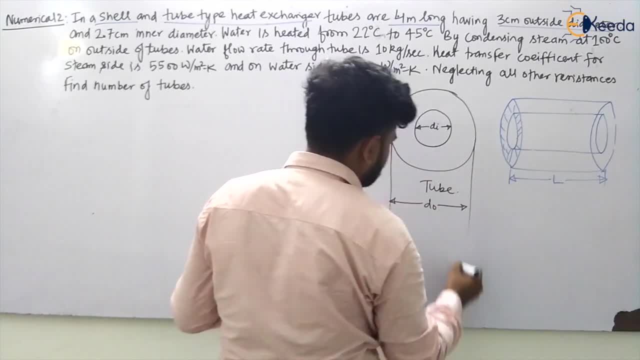 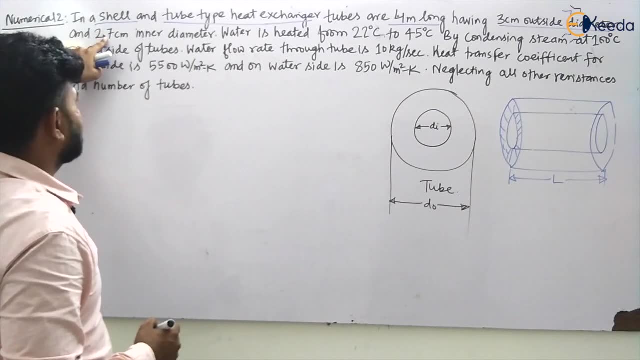 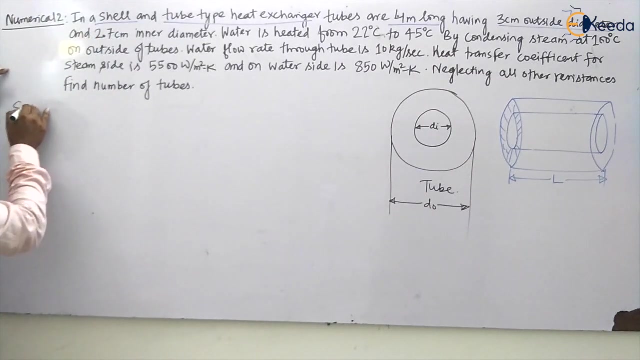 D0. okay, let us see now. and inner diameter is how much, having 3 centimeter outside diameter and inner diameter 2.7 centimeter. so your DI is given to be solution. let us your DI is given to be how much- 2.7 centimeter- and D0 is given to be. 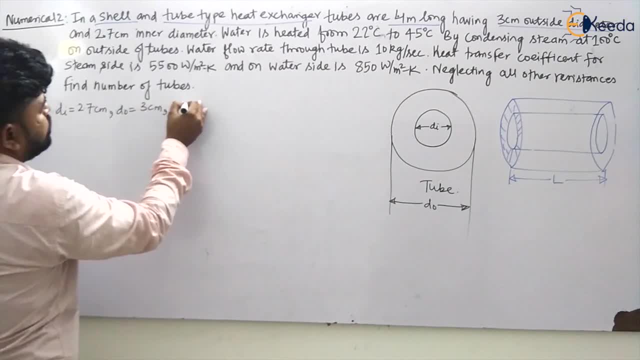 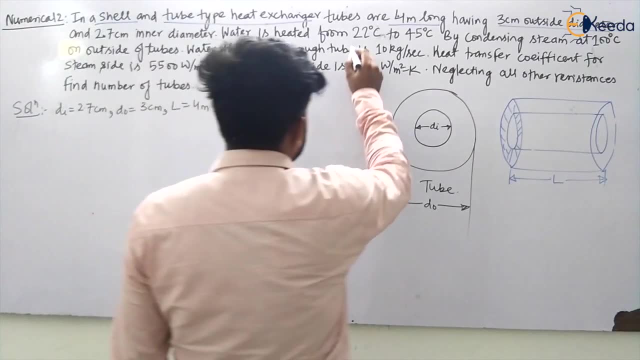 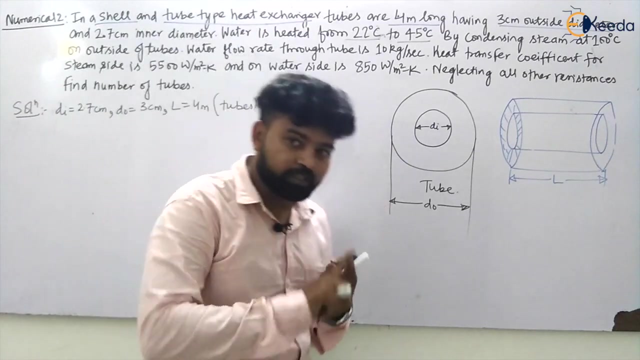 how much? 3 centimeter and length is 4 meter long, and this data is for tubes, my dear students, okay, now water is heated from 22 degree Celsius to 45 degree Celsius. okay, he is heating up water. he is heating up water from 22 degree Celsius to 45 degree Celsius by condensing. 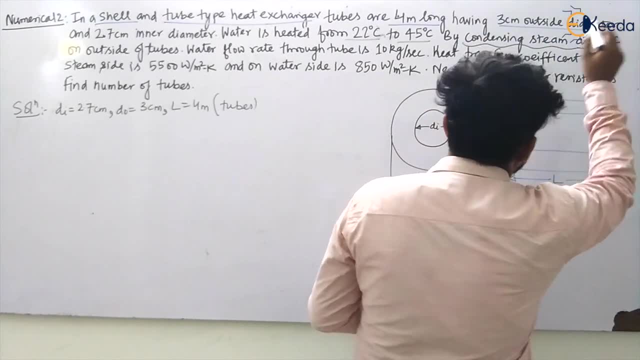 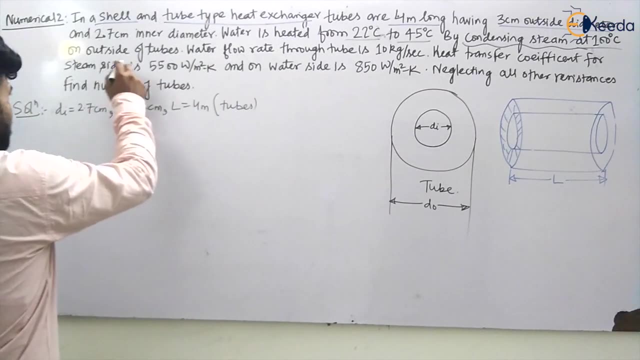 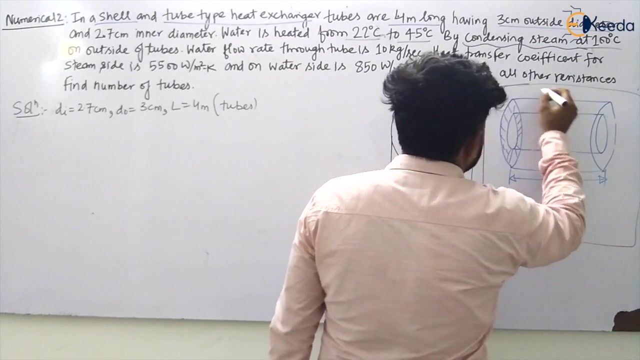 steam, okay, one is going to be like a phase change. one fluid is going under a phase change, my dear students. so steam at 100 degree Celsius, okay, on outside of the tubes, on outside of tube. so there is a in shell, it is, this tube is in Shell. so the steam is steam is there inside the cell. the 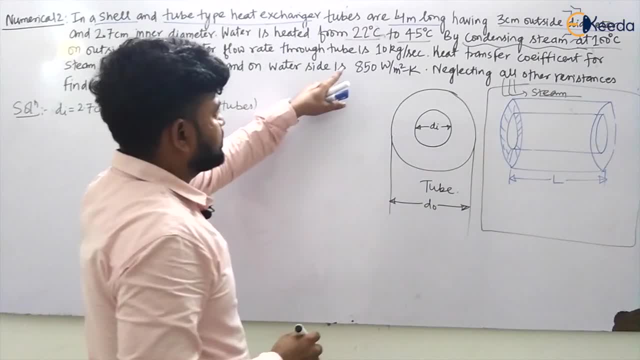 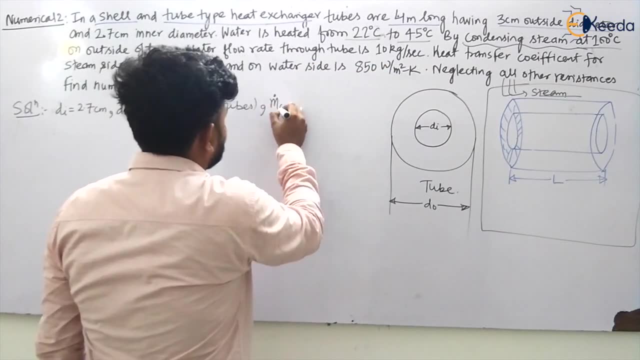 steam is forced, okay. the steam is forced through tube is okay. water flow rate through tube is 10 kg per second. so water flow rate is given, that is, of the cold flow rate is given to be 10 kg per second, my dear students. now heat transfer coefficient. 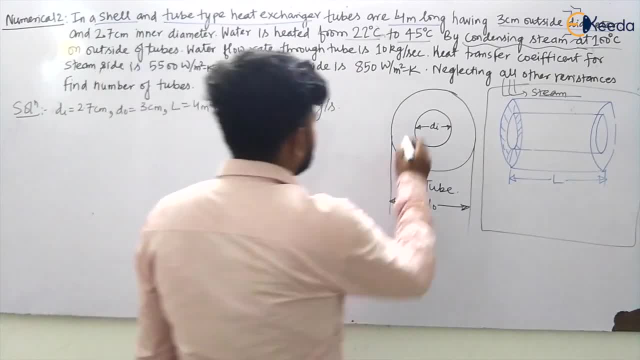 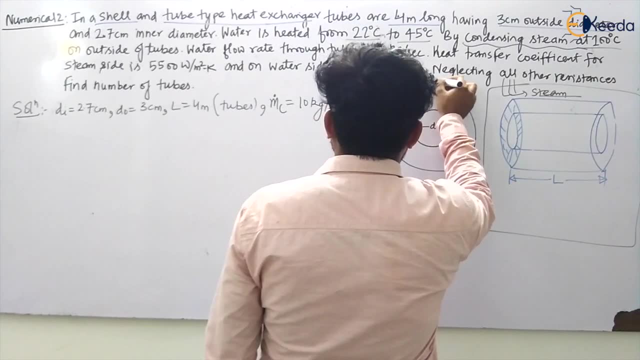 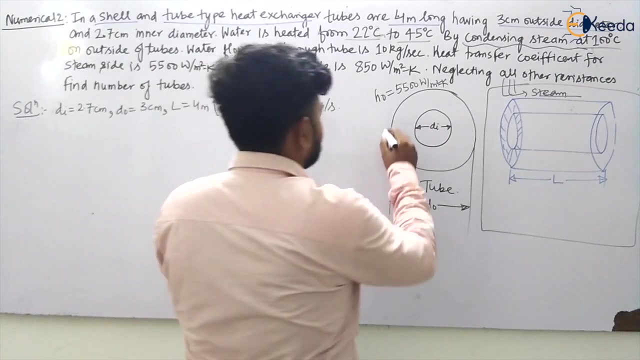 for the steam side is sufficient. 5500 degree Celsius, That is H. naught for the steam side is how much? 5500 watt per meter square Kelvin, And on the water side. on the water side means that is DI, So H. 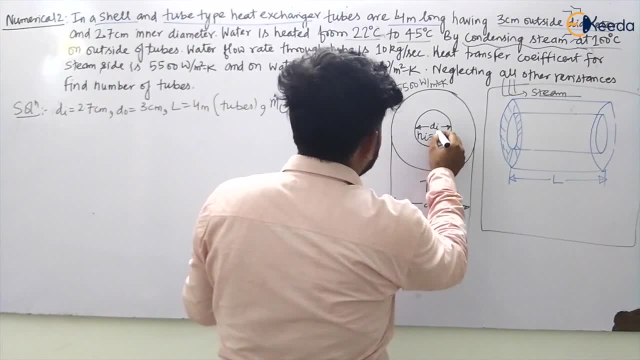 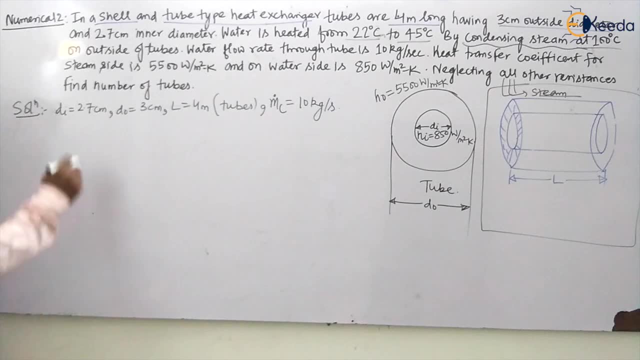 naught is given and HI they have given On the water side they have given to be like 850.. 850 watt per meter square Kelvin. Now electing all the other resistances, find number of tubes. So we have to calculate the number of tubes, my dear students, And he has given. 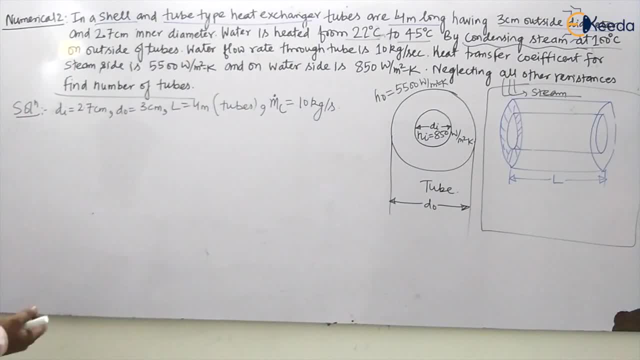 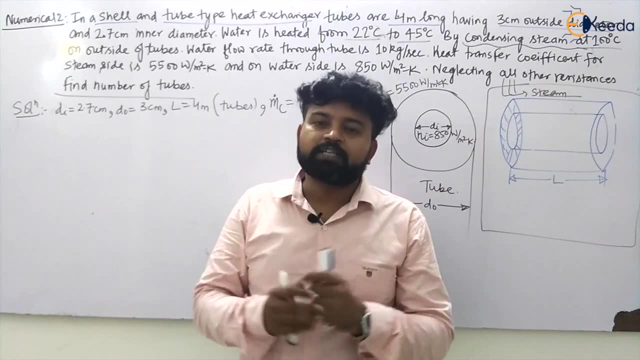 us which case. He has given us a shell and tube type heat exchanger which is undergoing a temperature change, And we know for a phase change heat exchanger we can easily calculate the delta Tm. Let us consider this case. So, if I will make the temperature profiles my, 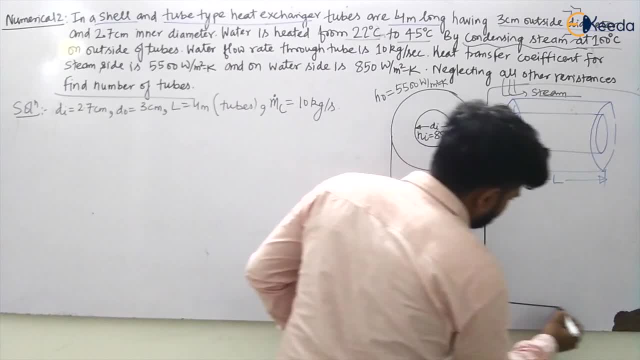 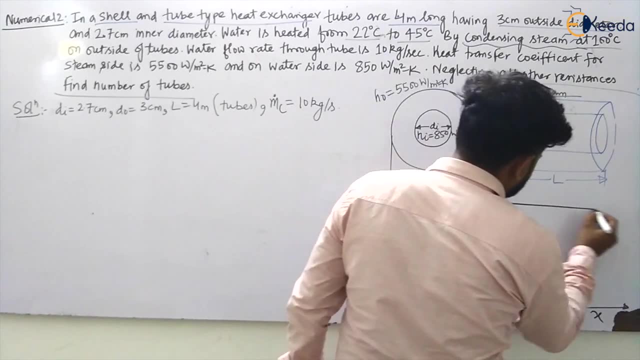 dear students, let us see what I will have. So one fluid is undergoing a temperature change. Let us take this is X, this is your T. So let us take this is your steam, which is at TH1 to TH2.. And let us take this hot. 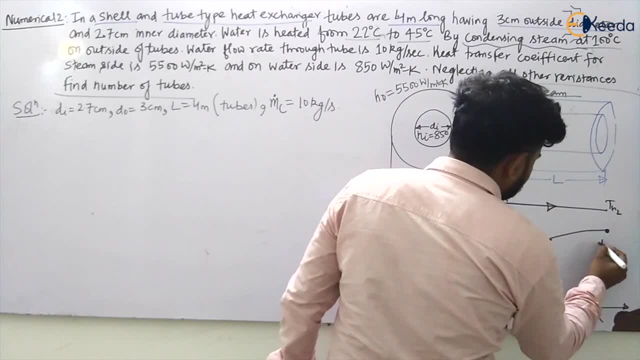 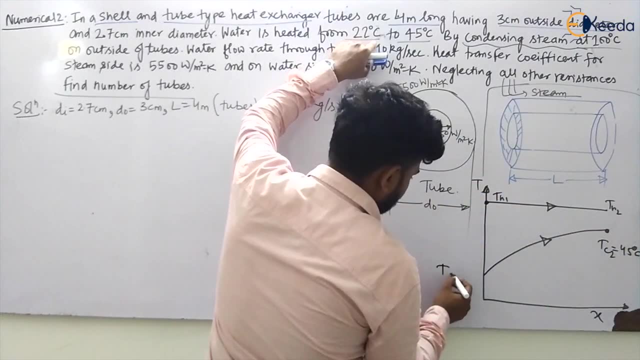 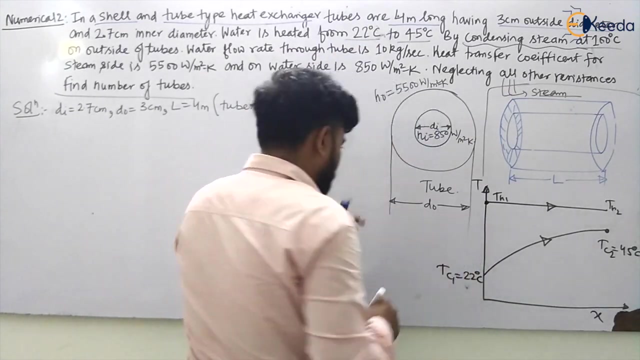 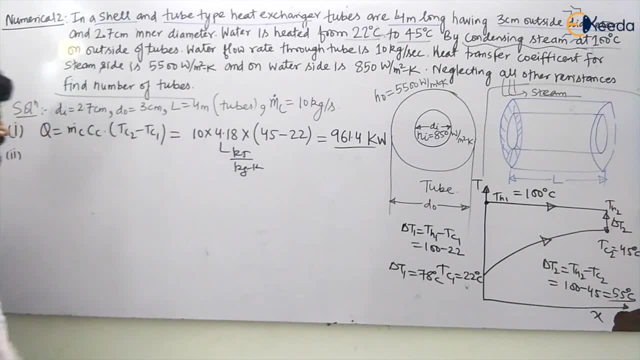 naught, So let us take this is H naught, So let us take this is H naught, So let us. and overall area of the heat transfer can be calculated by what? so they have given H0, they have given HI. okay, so can I have. can I have that overall area? yes, I can. 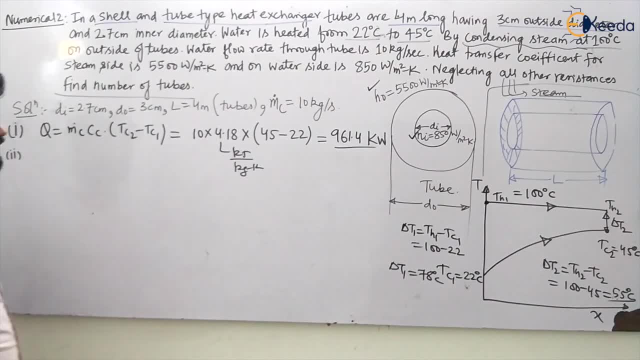 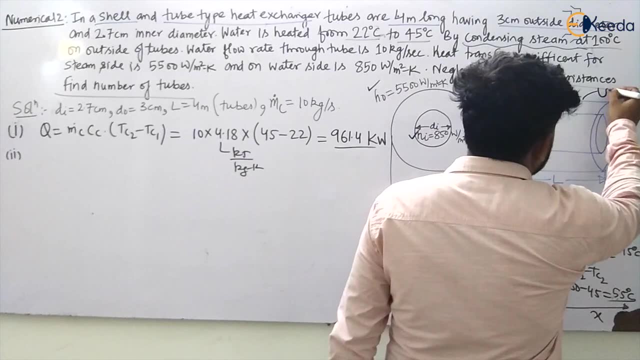 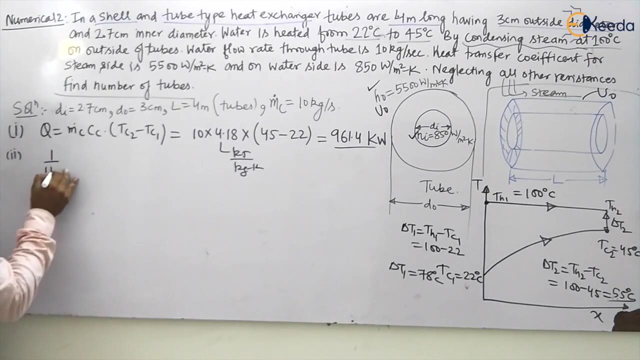 calculate that overall area, but how? first of all I have to calculate the. I have to calculate the overall heat transfer coefficient for the outside. that is U0 here. that is U0 here I have to calculate first. let us see how. so I want U0 to be calculated. 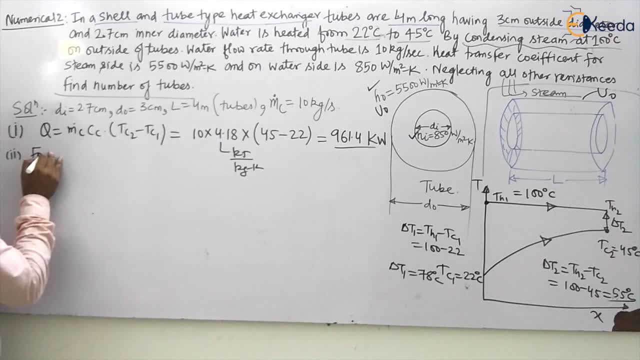 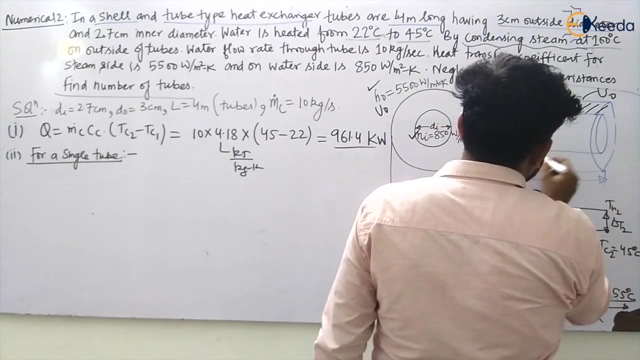 for the for a tube, that is, for tube for tube, for a single tube, for a single tube, my dear students, because I want to calculate outside, outside, if steam is flowing in this outside and this is your tube. so I want to calculate only U0, outside this. 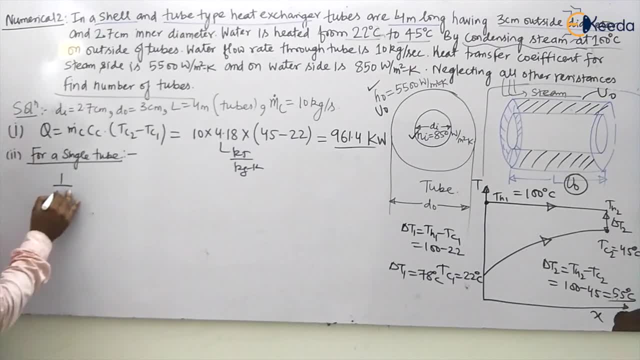 so this will be what this will be, even by. this will be even by. this will be even by: 1 upon U0 A0 is equal to 1 upon HI AI plus 1 upon H0 A0. my dear students, because what I have taken in this analysis, we have neglected the 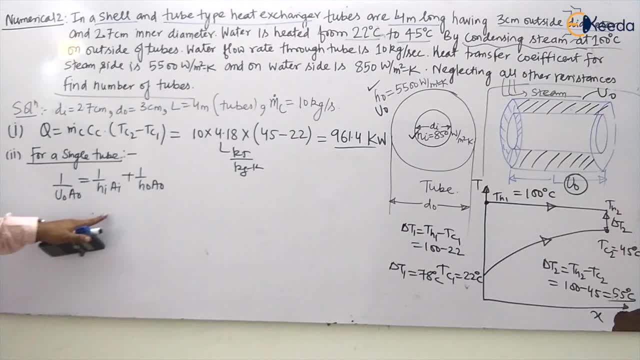 conductive resistance. so only I will take up to this, only my dear students. so this will become what if I will divide by A0, if I multiply both side by A0, so I will be having. I will be having what 1 upon U0 is equal to 1 upon HI AI. 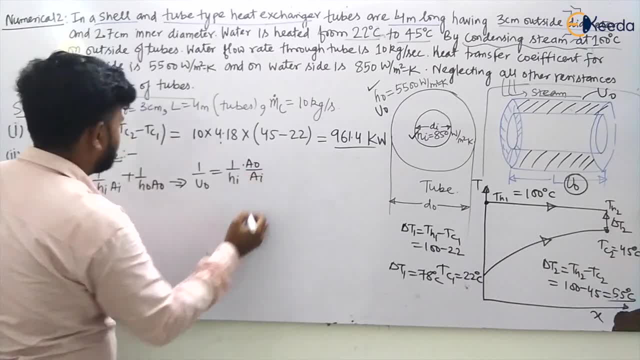 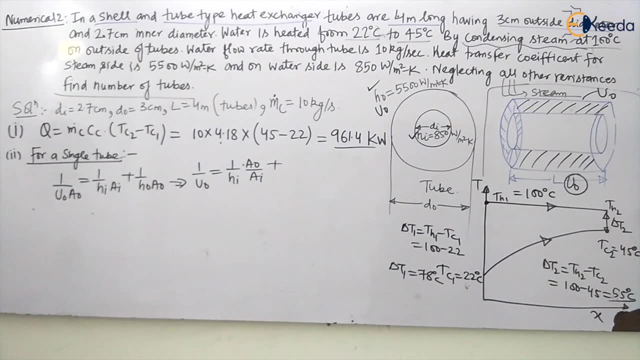 into a naught by a I, a naught by a i. plus let us take that to be like a small, a small, you know. let us say to be like small a naught, because I am taking for what I am talking. this will be small area, my dear students, for Q bank taking. 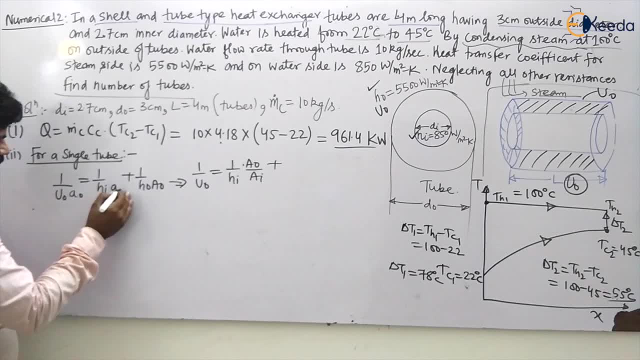 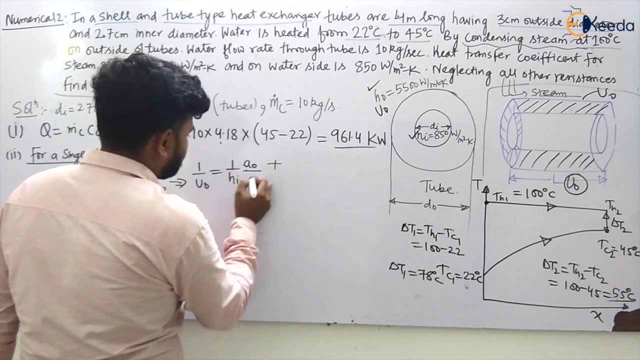 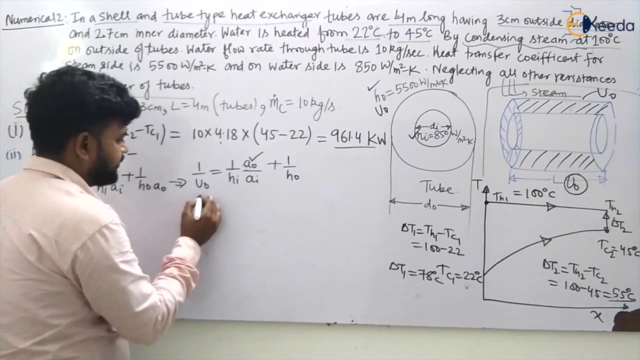 let us take it a note, let us take it a I. let us take it a. not of him. so again, I'm will have that A0 by Ai plus 1 upon H0. so what is the outside area of the tube I can write? so this will become equal to 1 upon. U0 is equal to 1 upon. 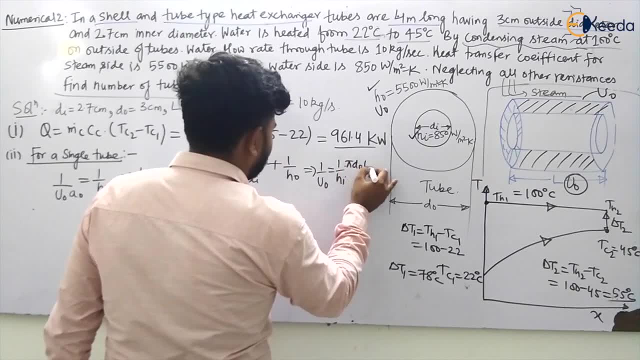 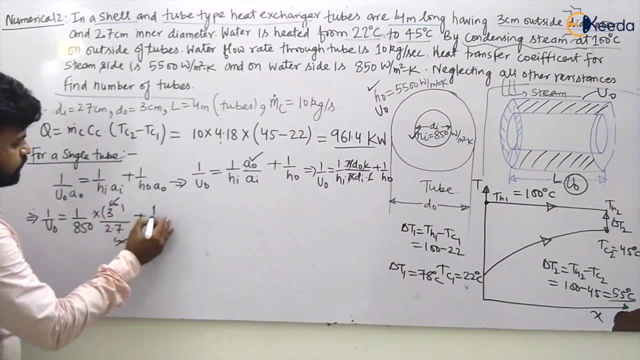 Hi into pi B0 L for that tube. if length is, L is the length of the tube. this will be in centimeter, centimeter. centimeter will go plus 1 upon H0, which is equal to 5500, my dear friends. so let us calculate this value. this will be 2.7. 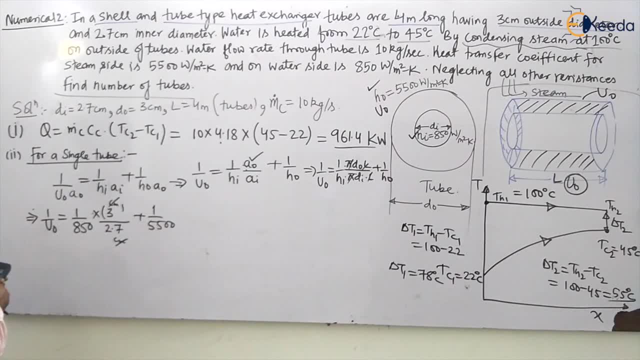 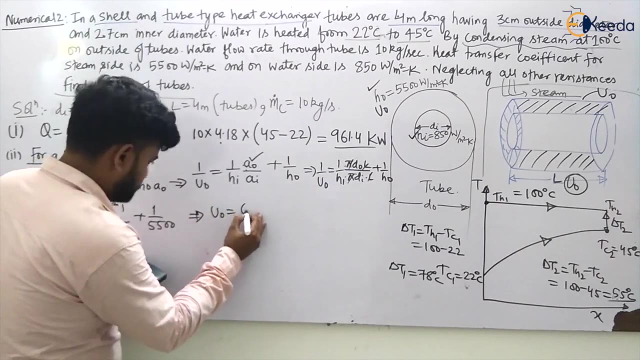 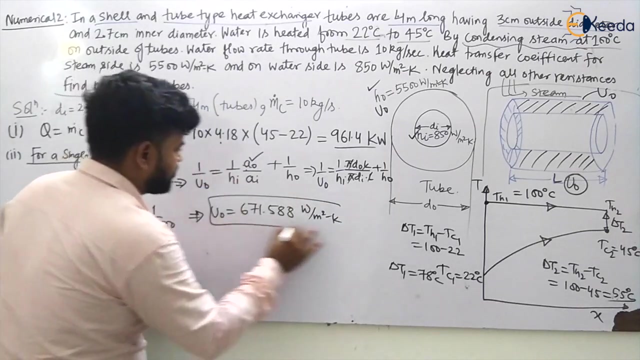 okay, divided by 850, plus 1 divided by 5500 and 1 divided by this, so I will be having that- U0 is equal to 671.58. that implies U0 will be equal to 671.588 watt per meter square, my dear students, watt per meter square, Kelvin. so now I have the U0 and I have 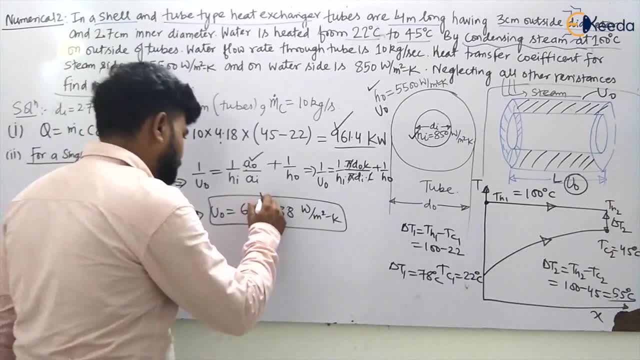 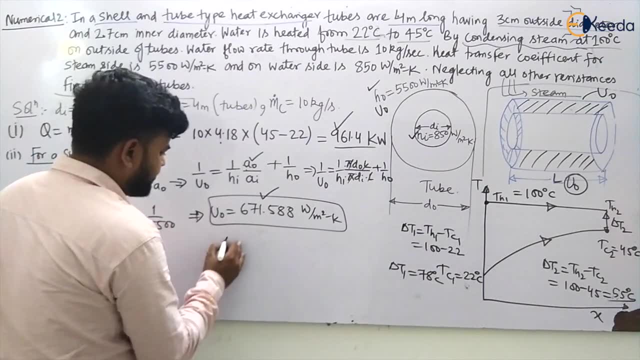 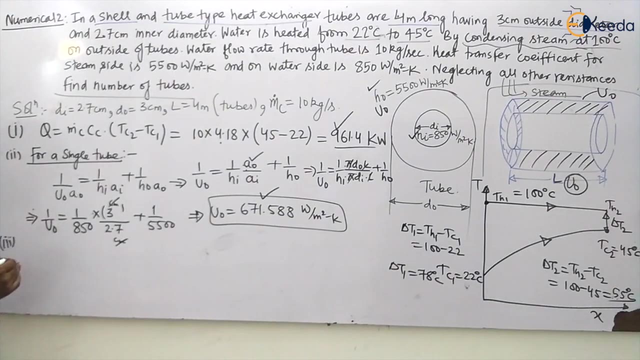 the heat transfer? yes, I have the heat transfer, I have U0 and do I have delta Tm? can I calculate delta Tm here? yes, what will be delta Tm? so delta Tm. let us take the third one. the third one will be: what delta Tm? so the third one will be: 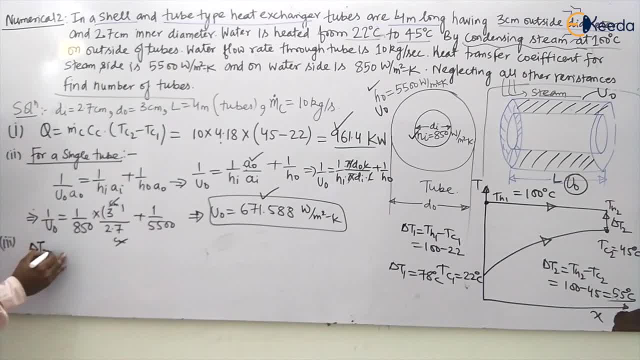 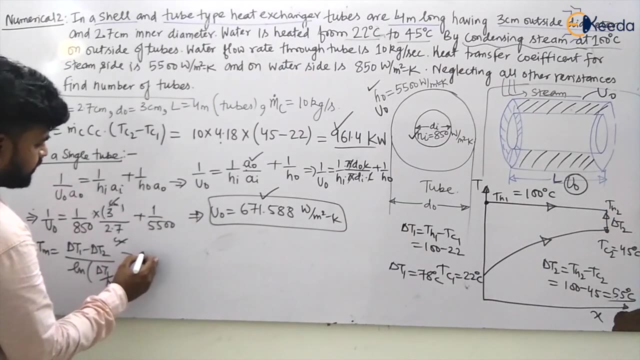 what delta Tm, my dear friends? so delta Tm will be given by delta T1 minus delta T2 divided by ln of delta T1 divided by delta T2. good, so delta T1 is how much delta T1 is? 100 minus 22, that will be your 78 minus. this is your, and this is your 100 minus 45. 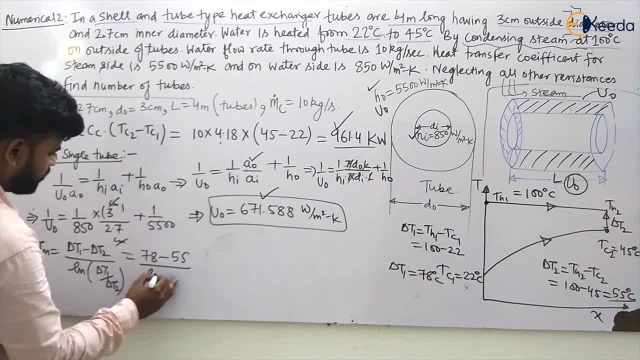 this is your 55 divided by ln of 78 divided by 55. so 78 divided by 55 ln, and this will be your 78 minus 55, my dear students. so this will be your 78 minus 55, my dear students. divided by this is this value will be 65.8, 65.8 degree celsius, my dear students. so now we know. 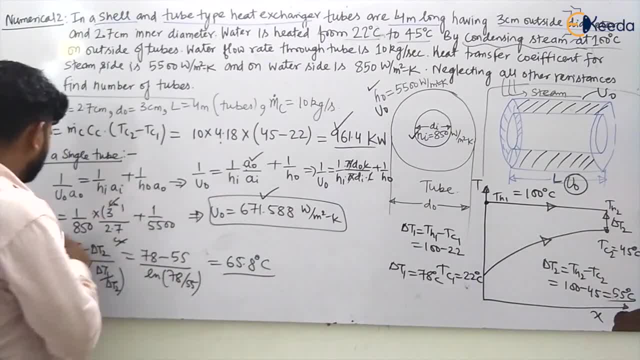 delta tm. we know delta tm also. now can we calculate the total area for heat transfer. yes, we can calculate the total area for heat transfer. so what will be? the total area for heat transfer is given by. the total area for heat transfer will be given by. let us see so the total. 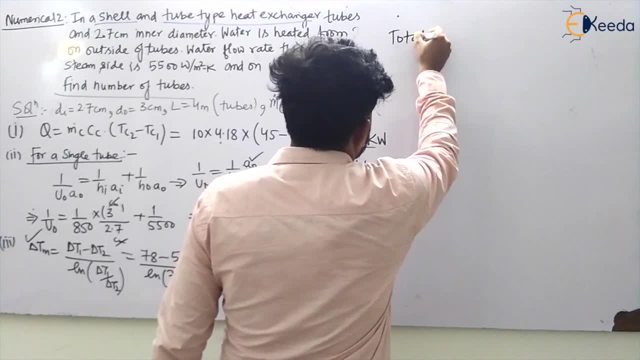 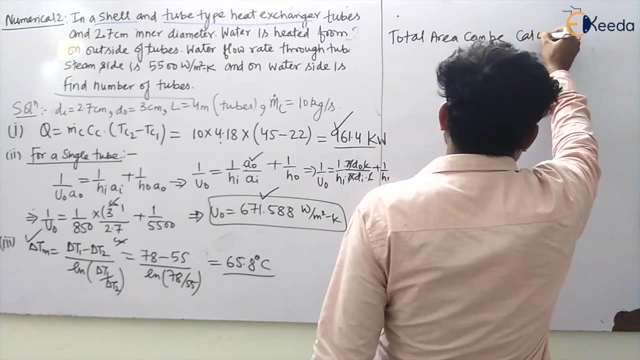 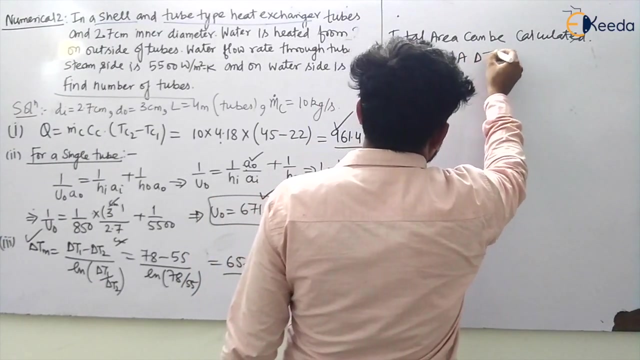 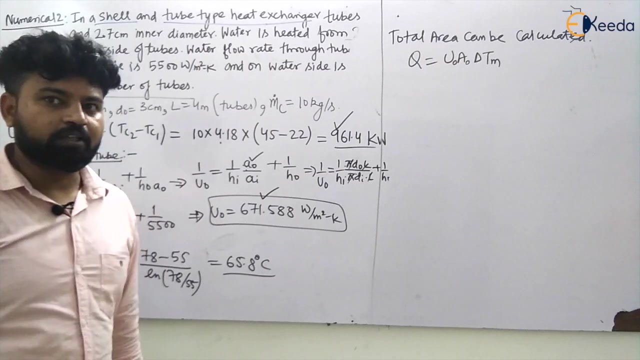 area area can be calculated, can be calculated. how this can be calculated, how this can be calculated? that q v no is equal to u, a delta tm, my dear students, and if we are considering the outside, then we will have only the outside area, we will have only the outside area. so q v no, how? 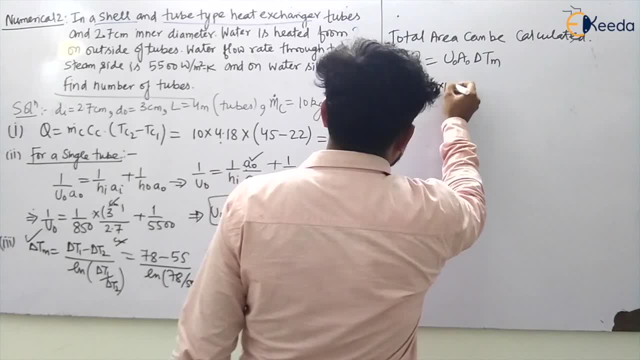 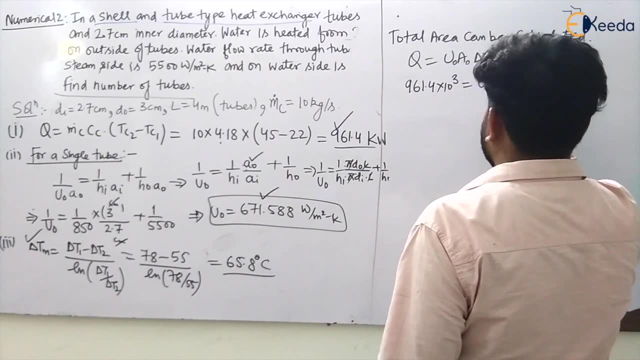 much is q, that is 3961.4 into 10 to the power of 3.. and u naught, we know now u naught is 671.588. my dear students, multiply by a naught, we have to calculate what is delta, tm, 65.8 degree celsius. so what we will have, let us see this- will be 671. 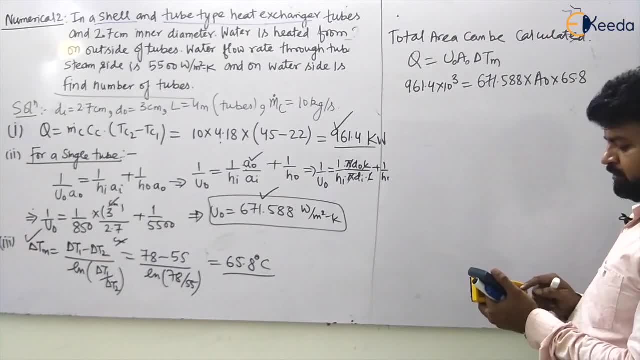 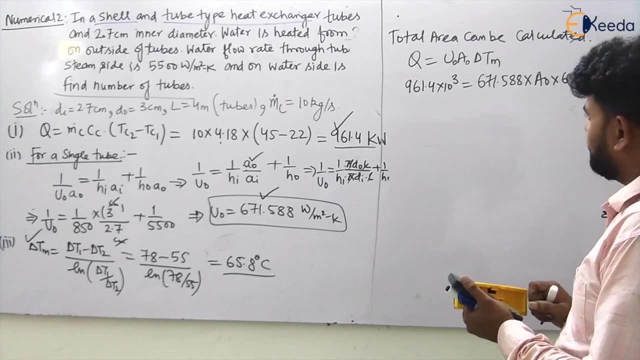 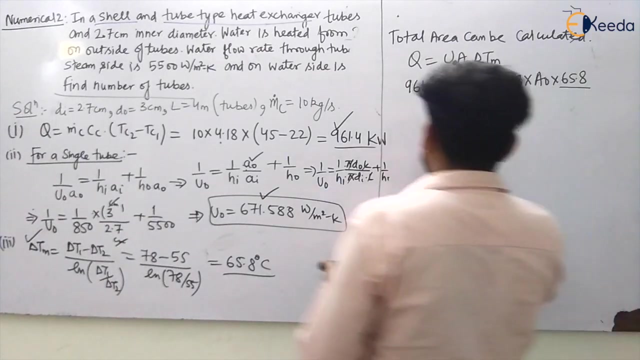 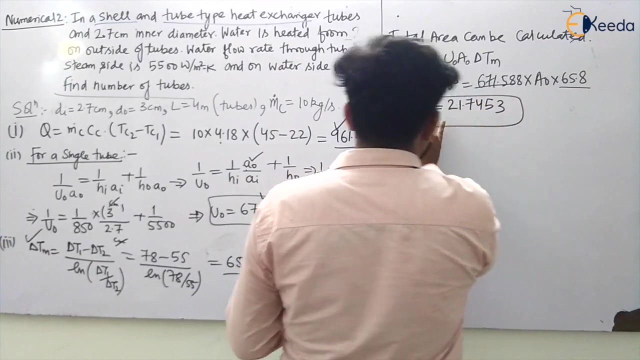 671.588, my dear students, 6715, uh, this, multiplied by this, okay, now 96, 961.4 into 1000, divided by this will be: so your a naught will become equal to 21.7453. so you know the total area now. you know the total area now. 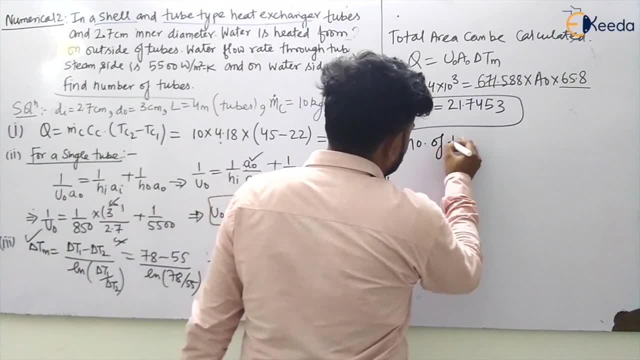 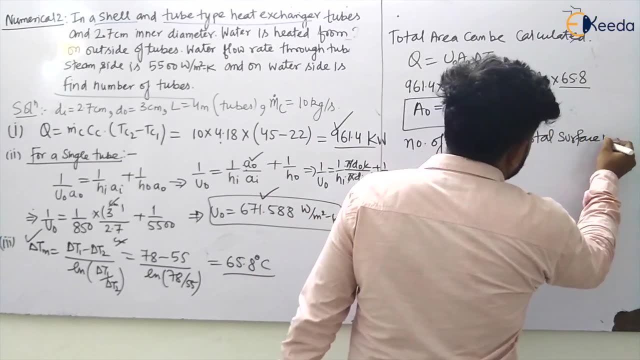 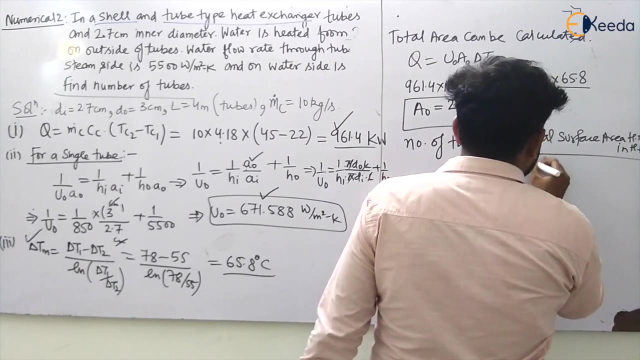 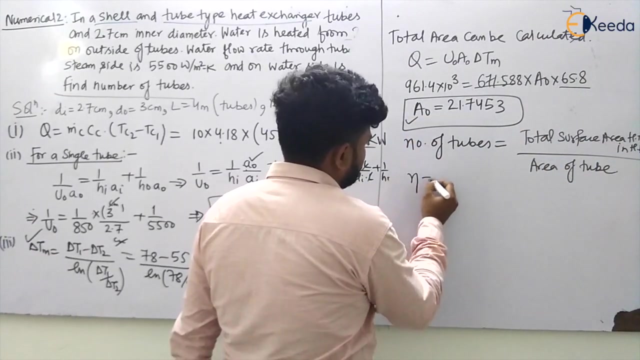 can we calculate the number of tubes? yes, number of tubes is equal to total area, that is, total surface area for heat transfer in heat exchanger divided by area of tube. area of tube. so this is your a naught, i will take a naught only. so this will be a naught upon a small 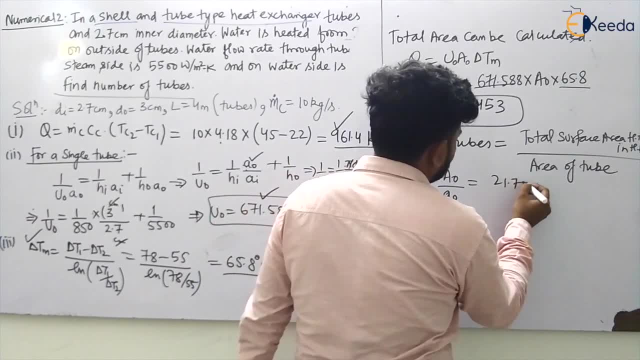 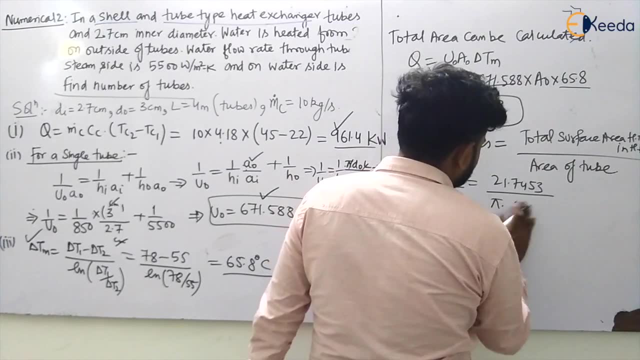 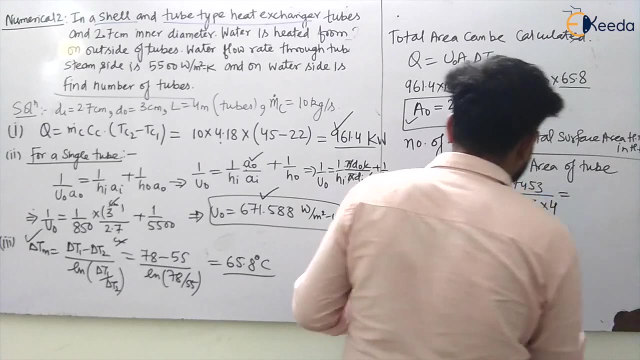 a naught. so this will become what? 21.7453. and what is the outside diameter they have given? pi? d is three centimeter. so this will be three zero point three. zero point zero three, my dear students. multiply by l, they have given it four. so let us see the. 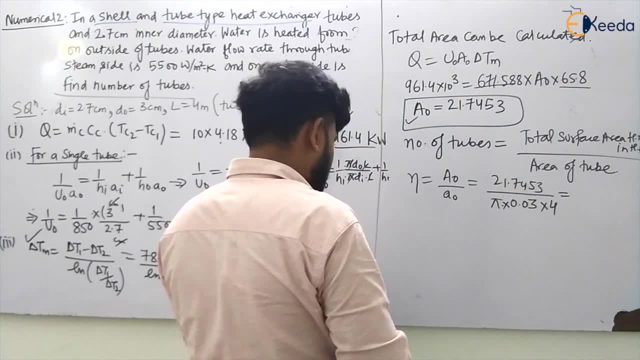 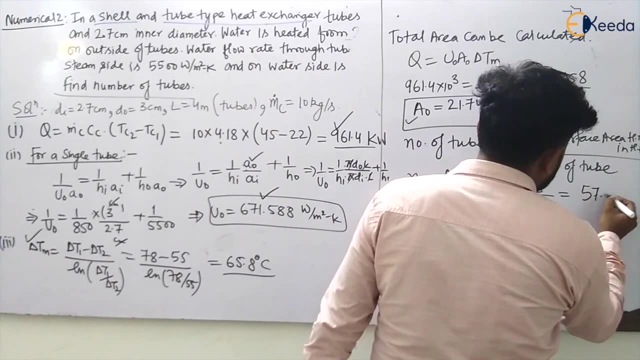 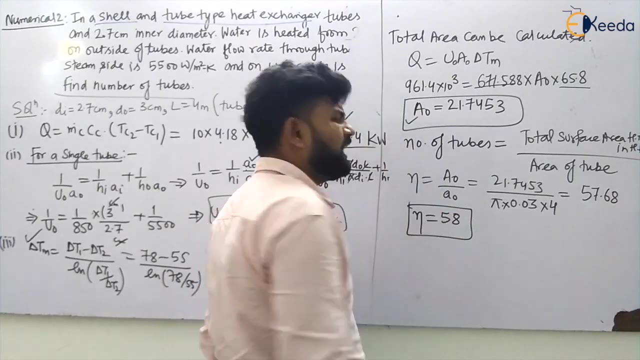 number of tubes divided by this, multiplied by 0.03, into four, so the number of tubes will be 57.68, my dear students. or we can directly take that n is equal to 58. so we have calculated the number of tubes by considering the outside diameter. so how many questions you have done? let us see. let us see. 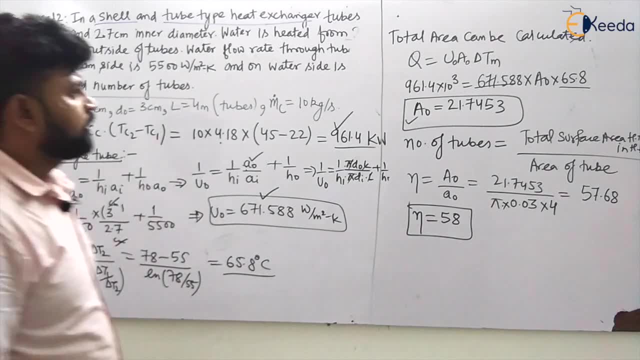 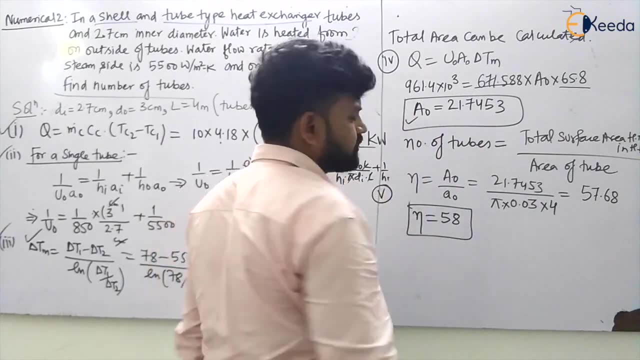 How i can calculate the initial diameter, Which is the combination of 1,, 2,, 3 and goes along the ratio of 8.. Again, you are calculating a naught. this will be like five, five questions you have covered in one population only and in the less time ideas. 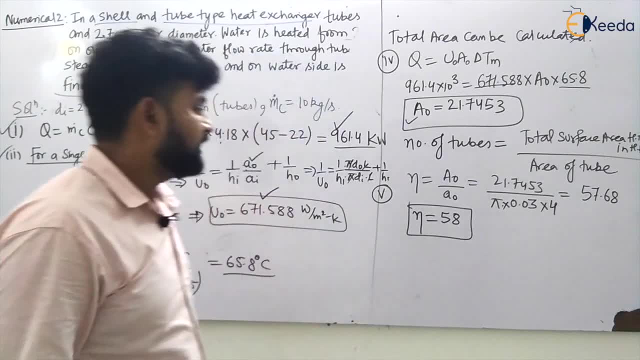 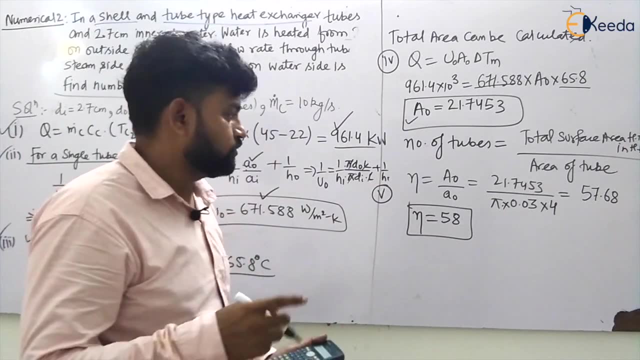 students and you have revised all the concepts. so calculate number of gestant into an ergonomic example. how many times creatinine is less other? Read up the special So you can calculate number of tubes on the basis of initial diameter, also by yourself, as now you know how I can calculate. calculate the initial. let us see the six one, six constant. 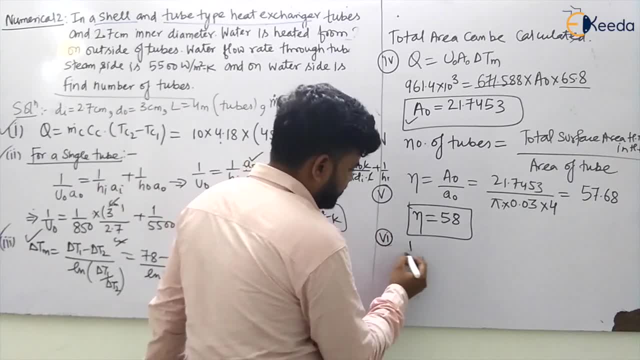 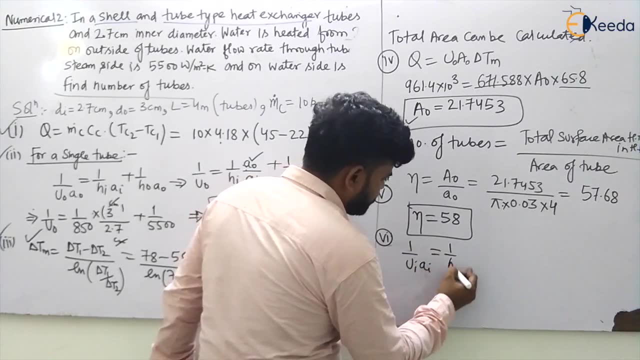 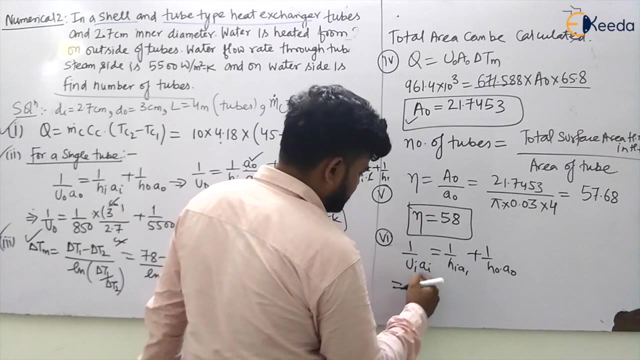 Let us see the sixth one, the sixth constant, 6th concept. so this will be 1 upon ui, ai. that is small. ai is equal to 1 upon hi into ai. for the tube i'm considering this will be 1 upon h0 into a0. so let us again do this: multiply with ai, both. 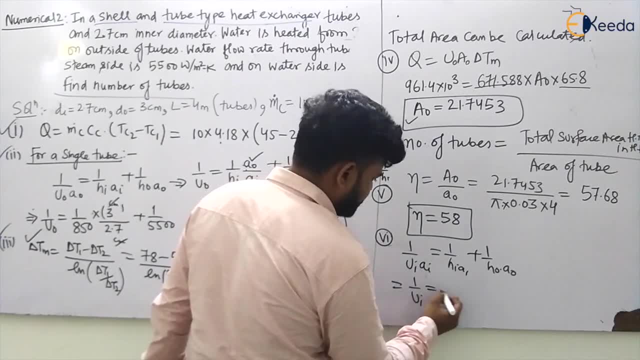 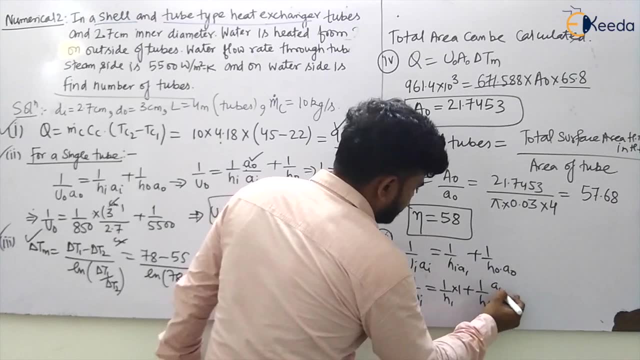 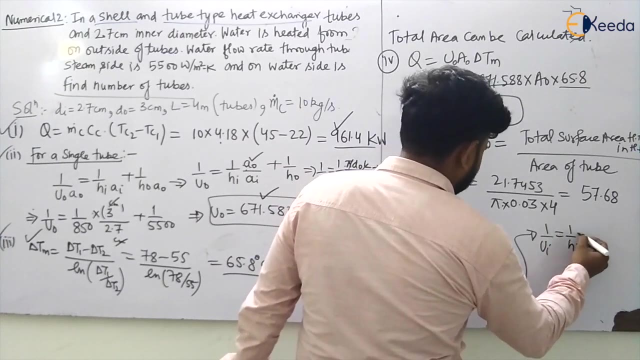 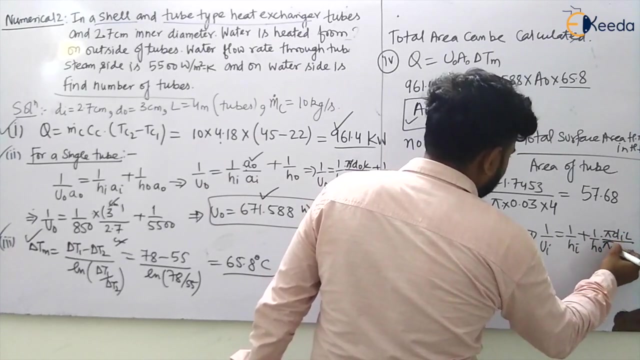 sides. so this will become ui- inner heat transfer coefficient, overall heat transfer coefficient: 1 upon hi, and this will become 1. now, plus, this will become 1 upon h0, ai by a0, my dear students, so we can write: 1 upon ui is equal to 1 upon hi plus 1 upon h0 into pi d, il divided by pi d. 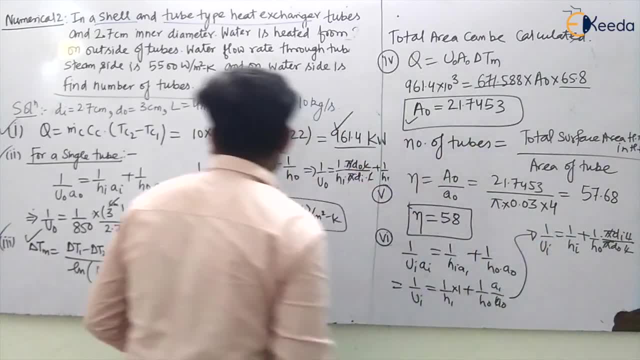 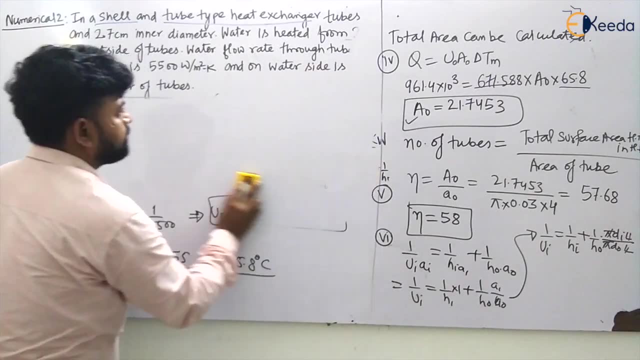 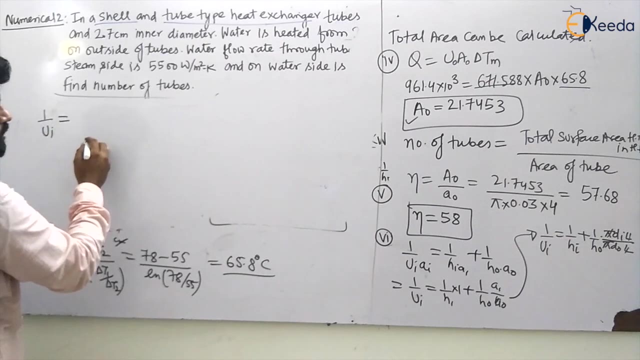 not l? l will go, pi, pi will go. so let us see what i will have. let us see, so, my dear students, in this case, what i will have. let us see. so this will become: 1 upon ui is equal to, is equal to 1 upon hi. what is hi, my dear students, so hi? he has given to be 850. 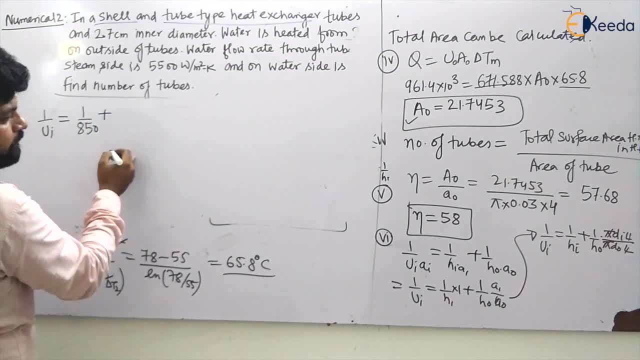 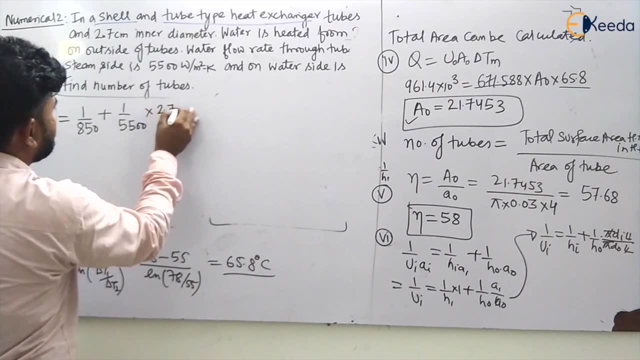 plus 1 upon h0. 1 upon h0 is how much? 5500, my dear students, multiply by di. he has given 2.7 d, not. he has given 3 centimeter. so centimeter, centimeter will go. so there is no problem. 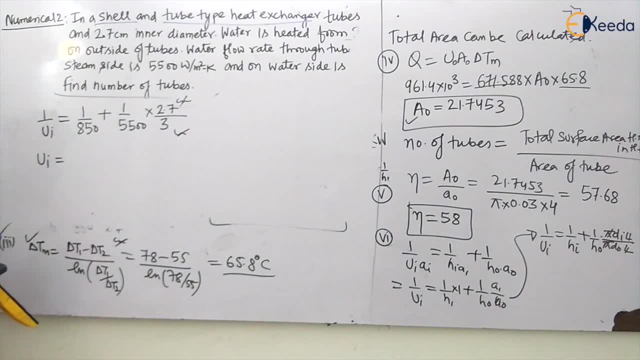 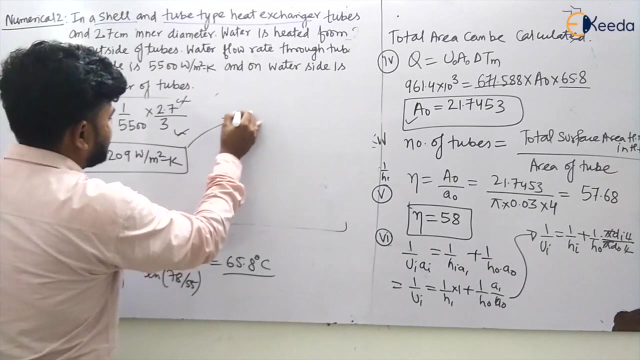 so let us calculate ui first. ui first. so 2.7 divided by 3 divided by 5500, plus 1 divided by 850- 1 divided by 850- he has got this- and 1 divided by this total value. so ui will be your 746.20, 9 watt per meter square kelvin. so we know ui, so we. 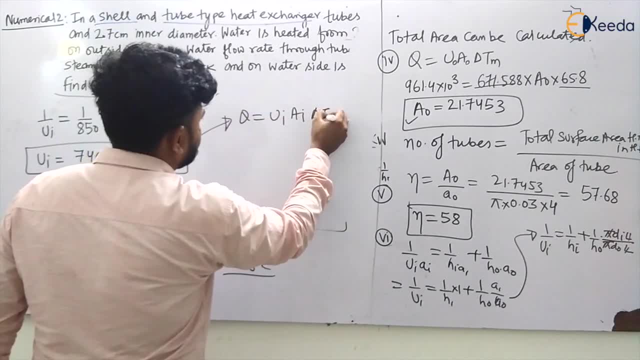 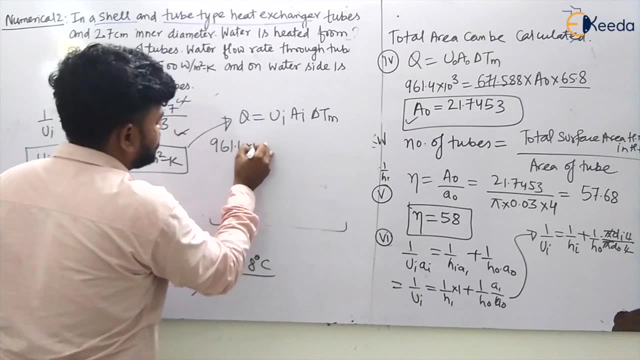 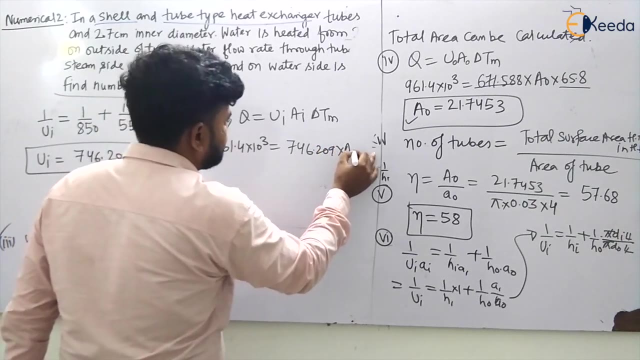 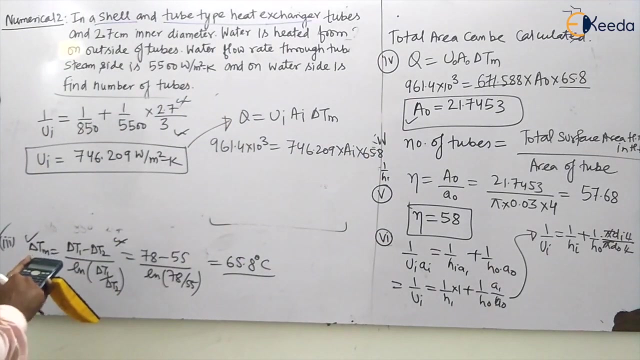 again that q will be equal to ui ai, delta tm. we know delta tm for all values. this is: that is 961.4 into 10 to the power. 3 is equal to how much 746.209 into AI multiplied by delta tm 65.8.. So let us calculate the values: 65.8 and that is. 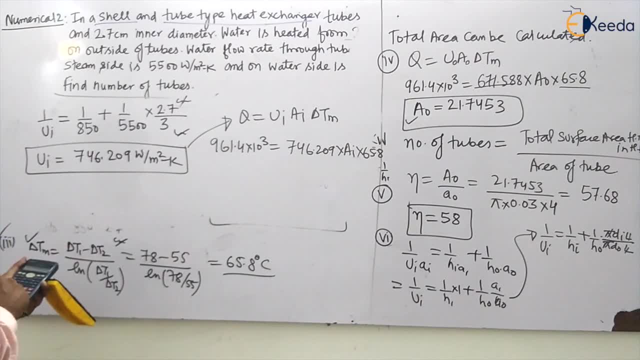 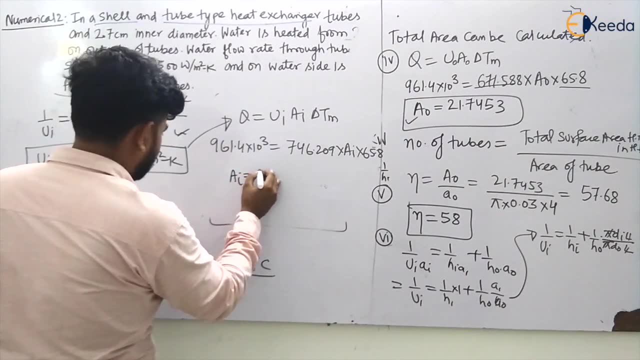 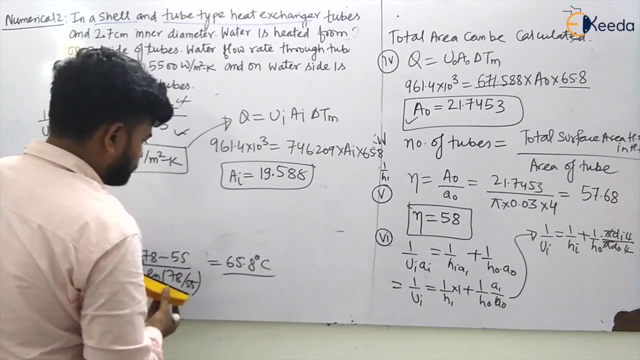 961.4 into 1000 divided by this, So we will be having the area equal to that is AI. inner area of the heat transfer. overall area for the heat transfer will be: AI will be this and number of tubes. you know, my dear students, will be given by what Number of tubes. let us see. 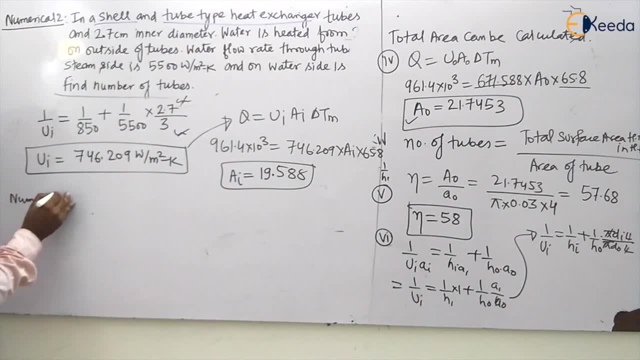 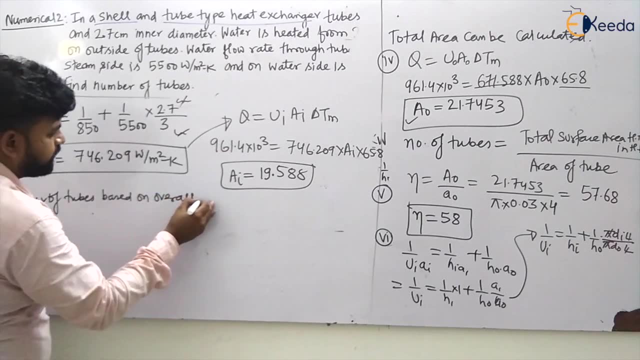 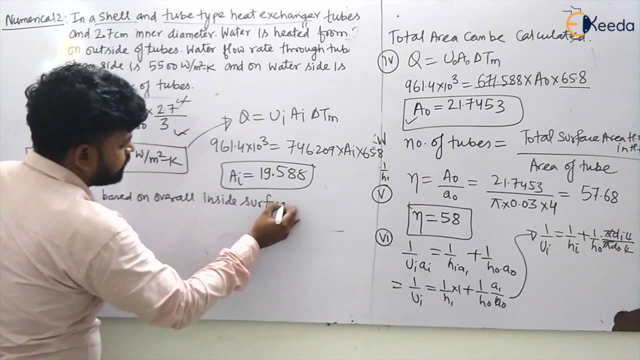 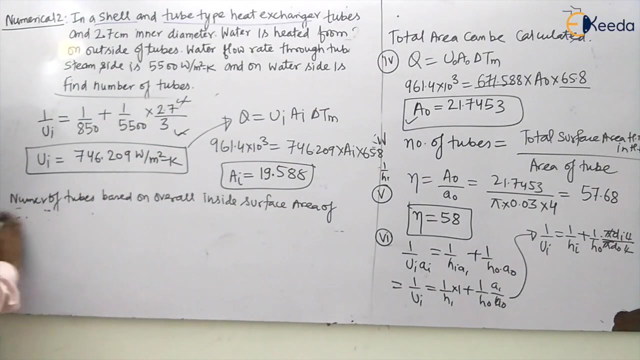 So number of tubes based on overall surface, overall inside surface area, inside surface area of tubes of shell or shell, we can say area will be given by what AI divided by small ai. So AI, we know 19.588,. my dear students, what will be small ai, Pi bi, which is 2.7 into 10 to the power minus 2. 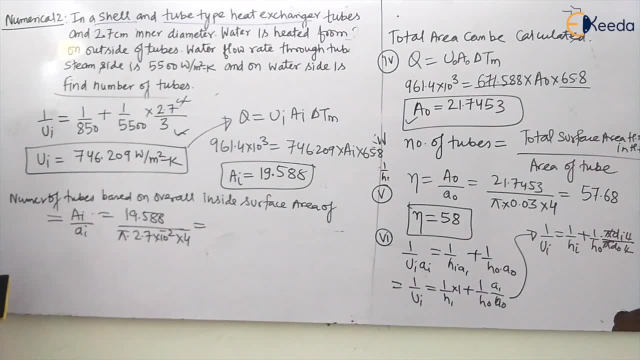 into L, which is 4.. So this will become how much, Let us see, Divided by pi 2.7 into 10, to the power minus 2 into L, which is 4.. So this will become how much, Let us see, Divided by pi 2.7 into 10, to the power minus 2, into L, which is 4.. 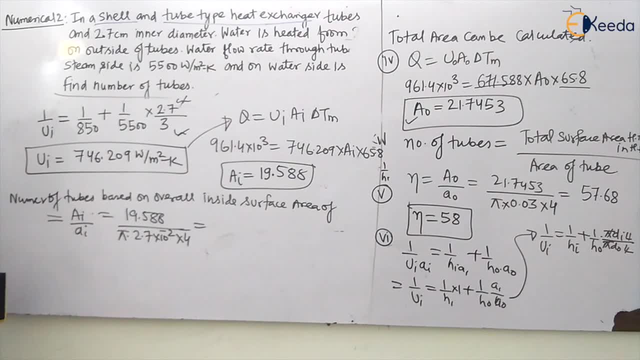 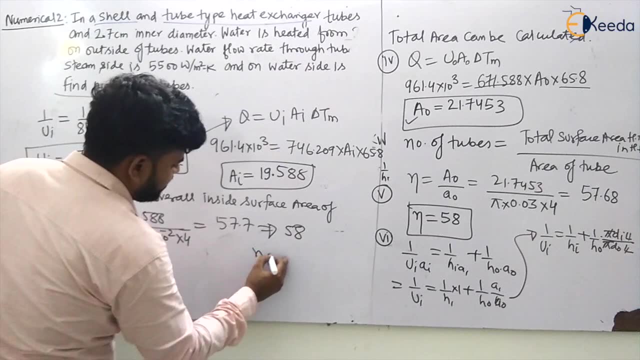 So this will become how much? Let us see: Divided by pi 2.7 into 10, to the power minus 2 into L, which is 4.. Divided by pi 2.7 into 10 to the power minus 2 into L, which is 4.. 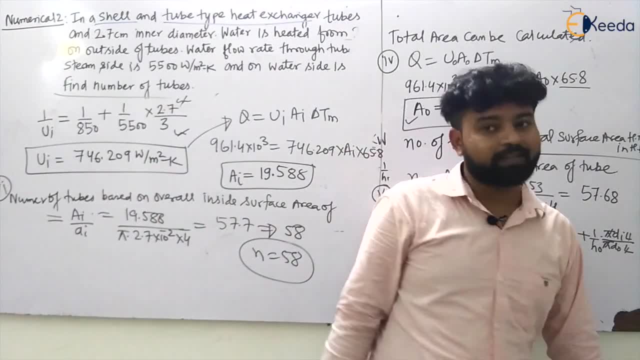 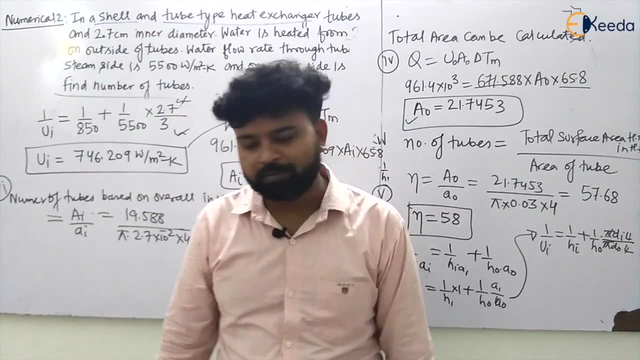 So this will be particularly important because we know that it is very small et So you will be taking that much in matter of seconds per second and letting it fight by itself. This will be 50You minus 2, multiplied by 4. 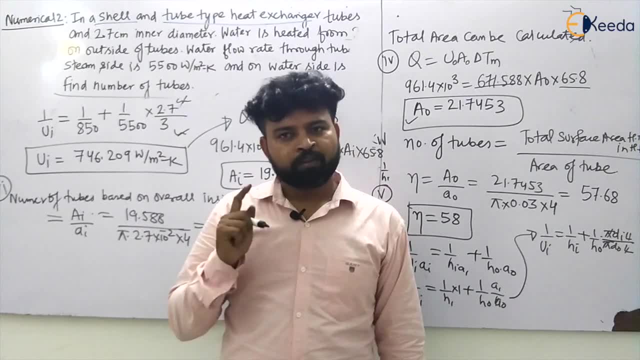 and again up to the concrete level. okay, hope you have understood the question. so, my dear student, thank you so much for this.